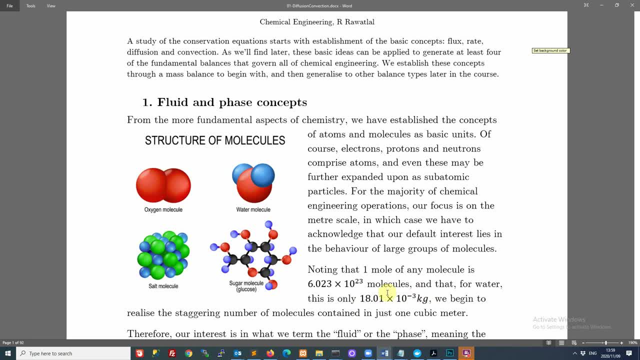 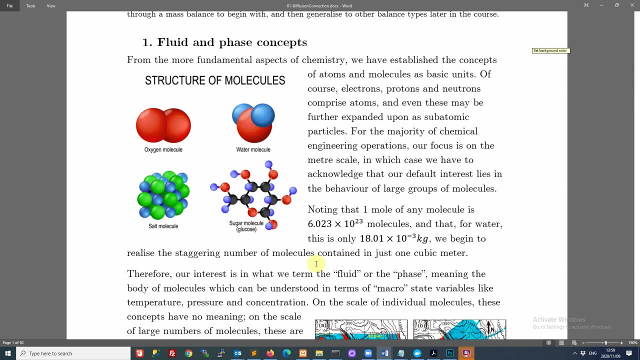 if you take just that number of that mass of a molecule of water that has 10 to the power, 23 molecules. That's an unimaginable number of molecules to us And in our chemical engineering systems. our interest is in the fluid or the phase. 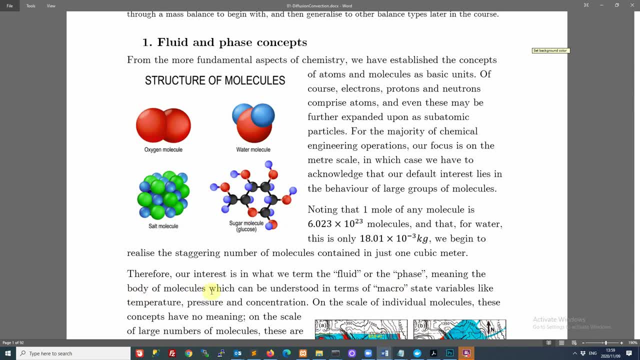 So by that we mean the body of molecules or the collection of molecules which actually describe the state of our system. So it might be a reactor or a distillation column or something like that, And our interest there is in how this fluid or phase is behaving. 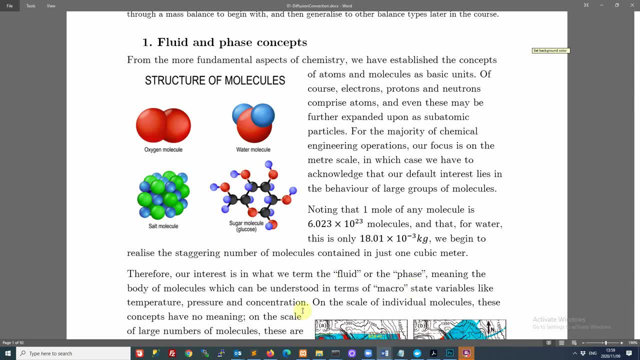 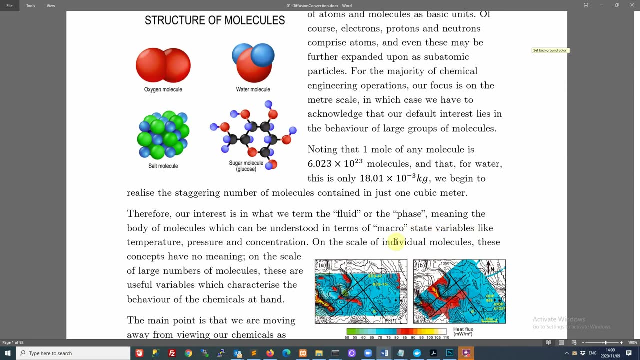 Now, when we say behaving, what we mean is the large collection of these molecules in that unit That is going to have a particular state, And so the state variables describe what form that phase is in. It's the form of the collection of molecules. 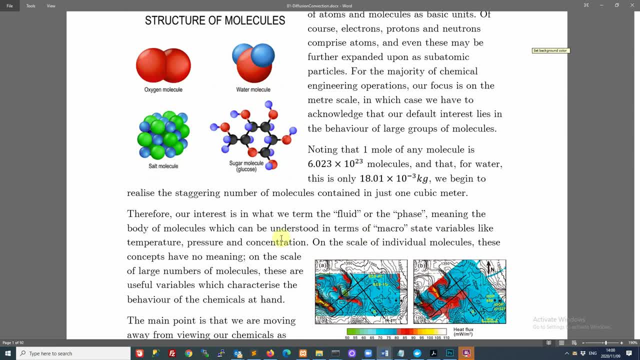 So we are talking about a large collection of molecules And the way we characterize the whole collection is in terms of these so-called state variables. So we can think about a temperature and a pressure and a concentration, And now these concepts are things we have proposed to understand how the group of molecules is behaving. 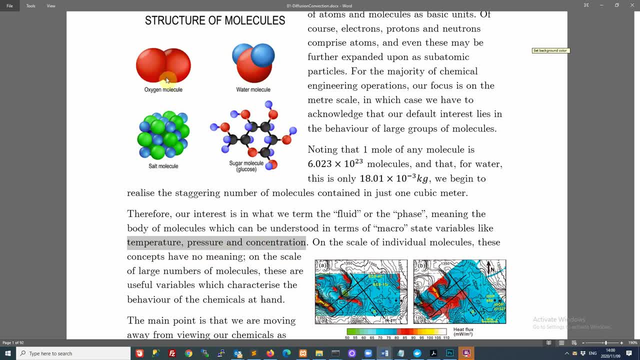 Right, These basic concepts do not exist in the context of an individual molecule. Remember, temperature is the average condition. Temperature is the average kinetic energy of molecules. So if you look at a single molecule, we can't really talk about the temperature of a molecule. 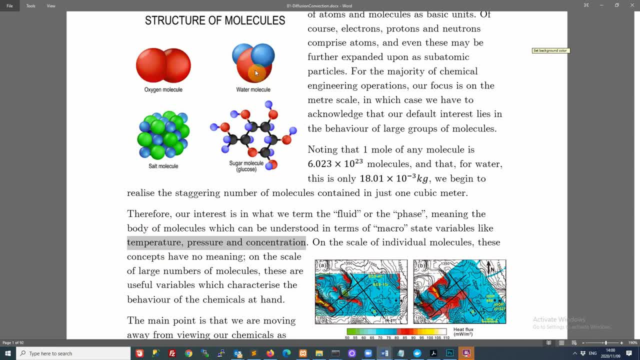 It's the average state of vibration of all the molecules together that gives us what we experience as temperature. And we have to acknowledge here there is some human bias When we stick our hand, for example, in some fluid, into a tub of water for instance. 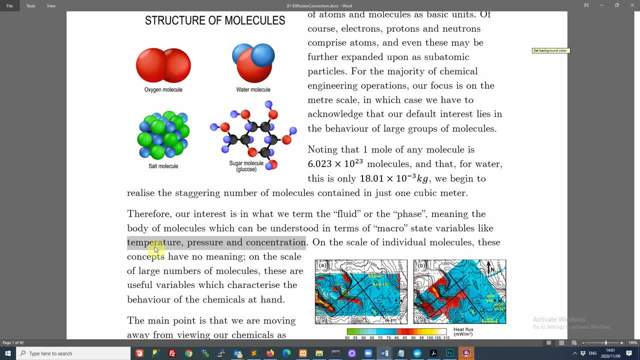 we experience temperature in terms of the level of pain, according to our nerves. So our nervous system gives us some impression: Yes, this is hot or no, this is cold. So we understand temperature because that's the scale that we live at. 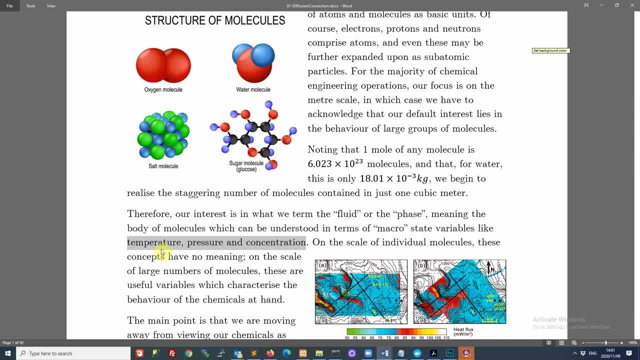 We live in the cubic meter scale, if you like. Now molecules are living in a much smaller space than that. What we experience as temperature is actually the collection of molecules. What we experience as temperature is actually the collision of many, many molecules. 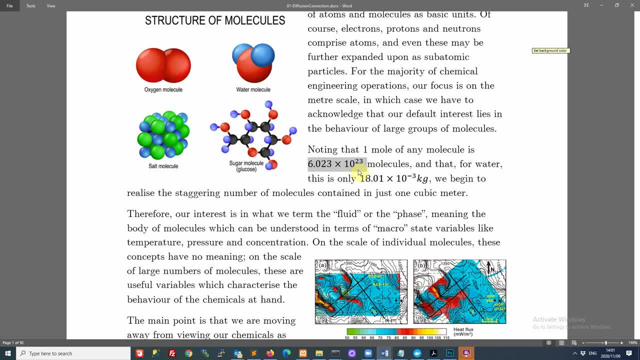 an incredibly large number of molecules, an unimaginably large number of molecules. So the collision of those molecules against our nervous system is what we experience as temperature. So the concept of temperature doesn't exist in the context of a single molecule. A single molecule vibrating- we might do something like estimate its average vibration. 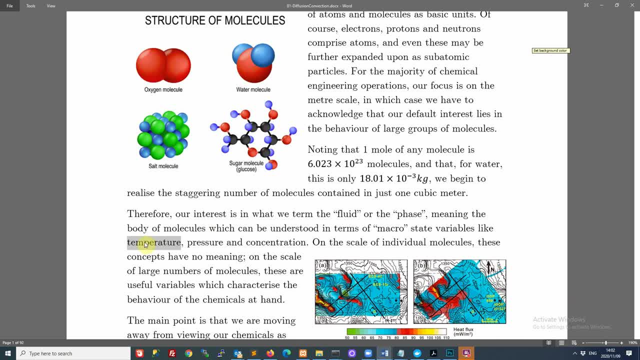 over time or something like that. but what we experience on the cubic meter scale is quite different to what's happening at the molecular scale. Similarly, the influence of pressure- what we call one atmosphere of pressure- is actually the repeated collision by an incredible number of molecules. 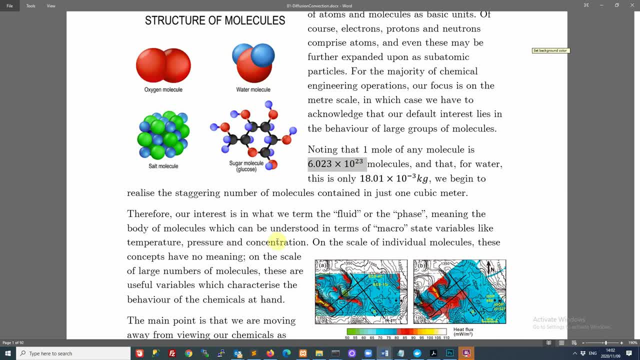 against some measurement device. Similarly with concentration. if we talk about a concentration of 2,000 moles per cubic meter, that is again an incredible number of molecules that exist within one cubic meter. So these are macro state variables. 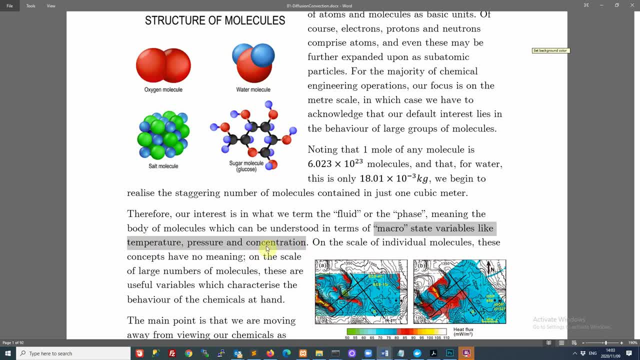 And so these are characteristics, these are variables that we use to summarize the state of our fluid. So when we talk about a fluid, we are talking on a much larger scale than individual molecules, And if you think about, for example, a weather pattern, 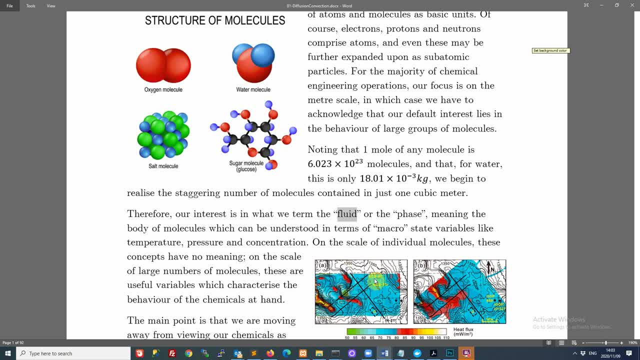 when we talk about a temperature distribution across a country. that is a good example of our interest in how the state of a fluid is varying across a space, And an important thing to notice here is that we are thinking of this as a continuous phase, when, in fact, when we zoom right into it. 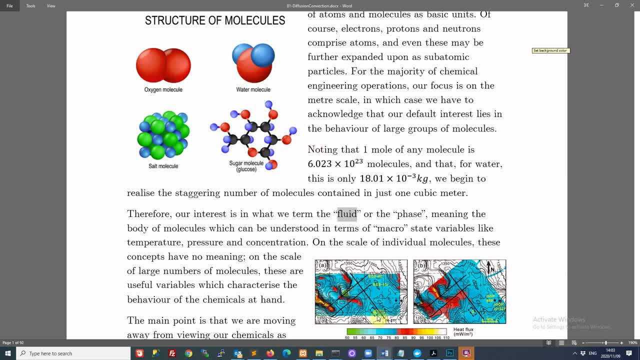 we see individual molecules. So we treat a fluid as a continuous phase, with the understanding that because we have so many contributors to that space that it starts to look as if it's a continuous body, whereas in fact it's comprised of these discrete elements. 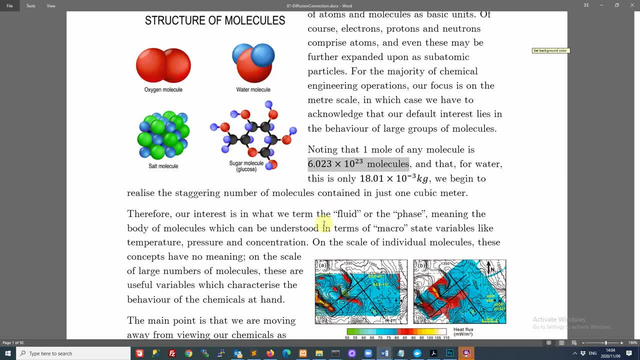 So these are all distinct elements, whereas we treat the large collection of such elements as a continuum and a phase, And we can generate maps like this for any phase variable. So, for example, in a weather pattern, we often talk about the temperature distribution over the space. 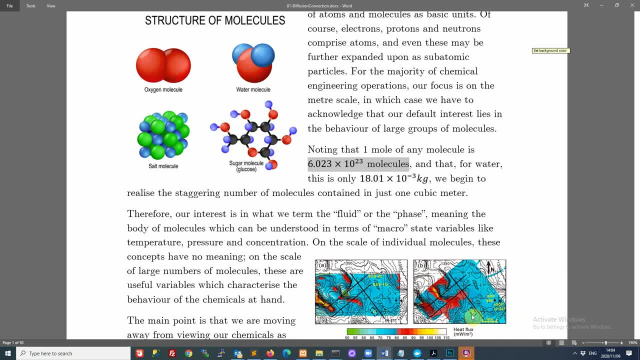 and we know that that distribution changes over time. So on one day this might be a temperature distribution, On the next day the red areas may have shifted to other places on these axes and so on. So the state of the phase changes over time. 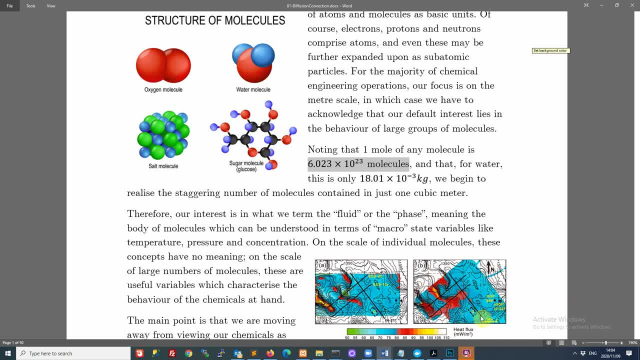 And we can draw such a picture for any state variable. So we've mentioned temperature. We know that we can generate such a picture for concentration as well And, of course, in terms of the weather, we don't really talk about concentration. 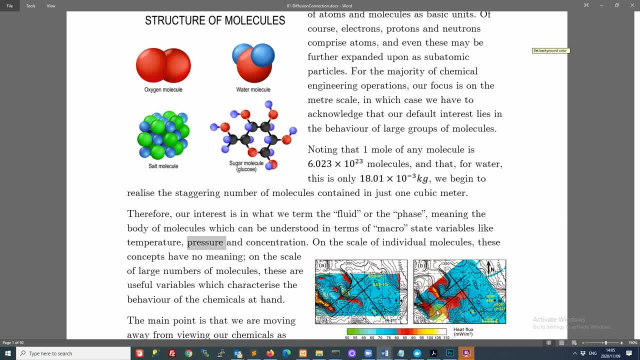 Number one. there's a very small variation in the air concentration over such large volumes, But in our chemical processes we are more interested in how the concentration varies. It might well be the case that, for example, the concentration at the inlet point may be very different. 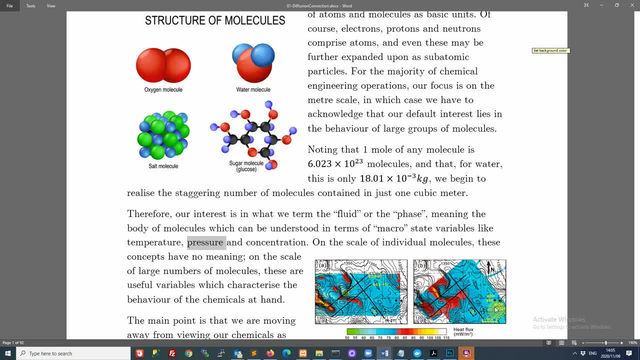 compared with the concentration at the exit point, if this was a map of some vessel. And the same applies to pressure. We can draw such a picture for pressure. We can also draw such a picture for velocity, And in the case of velocity there are more states of interest. 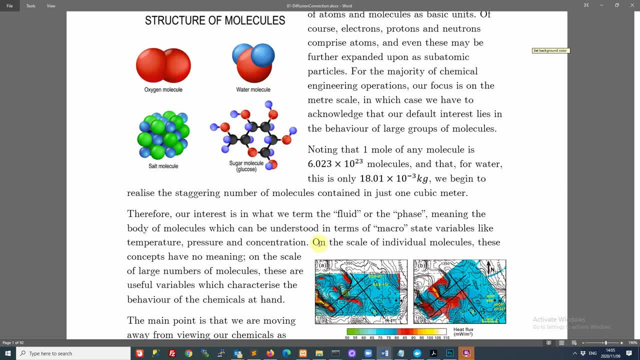 So in the case of velocity, the velocity vector describes how the fluid is behaving in all directions. So, for example, if we have a velocity vector pointing like so, then that's telling us there's a certain magnitude that the fluid is moving in this direction. 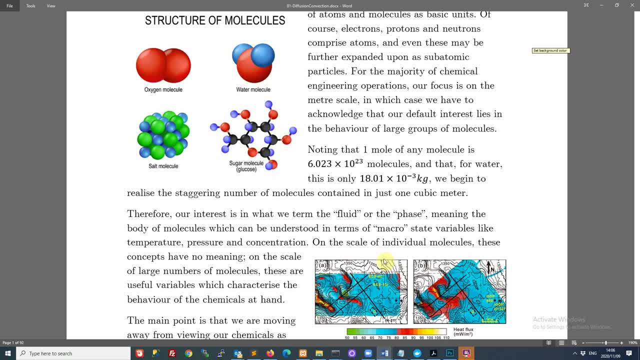 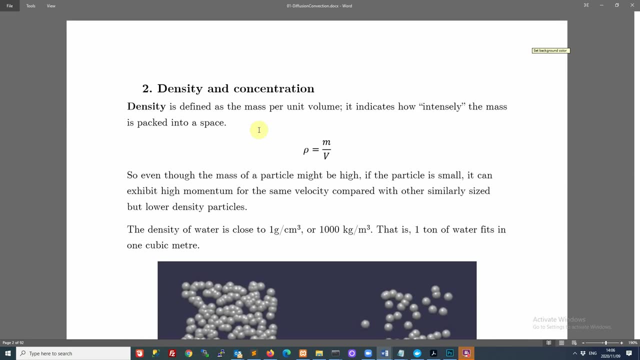 and a certain magnitude, that it's moving in that direction. So we start to view our fluid state as something that's distributed over space and across time, And so we can say here, for example, if we are talking about density and concentration: 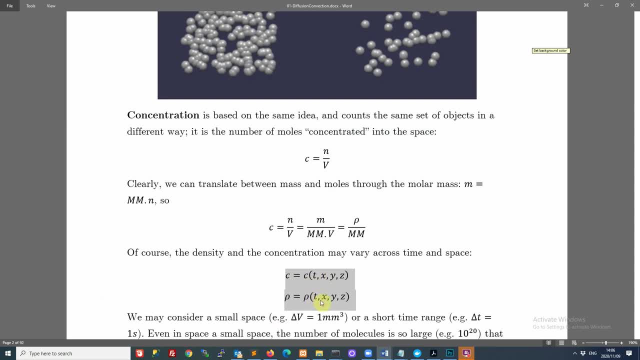 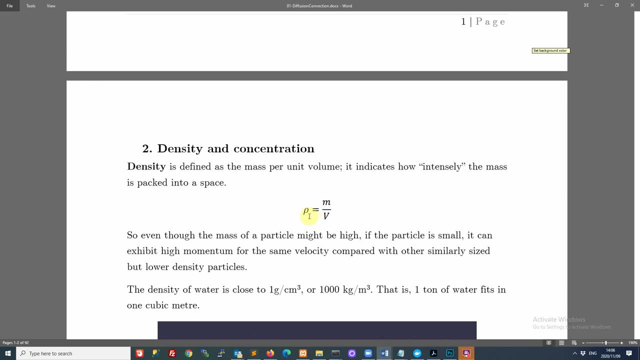 density and concentration are varying in both time and space, And so here we are introducing more of these fluid variables, So we can talk about the density of our fluid as being the mass of some volume divided by that volume. So that is an indication of how tightly packed the molecules are in that fluid. 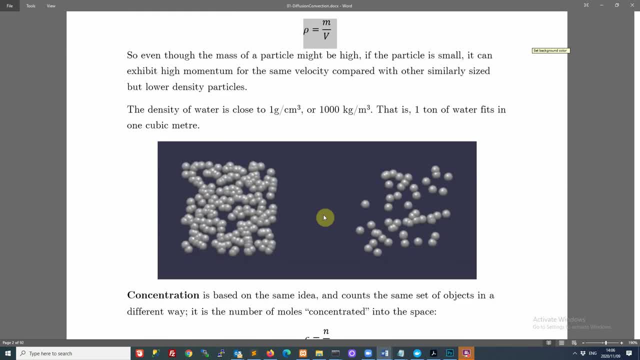 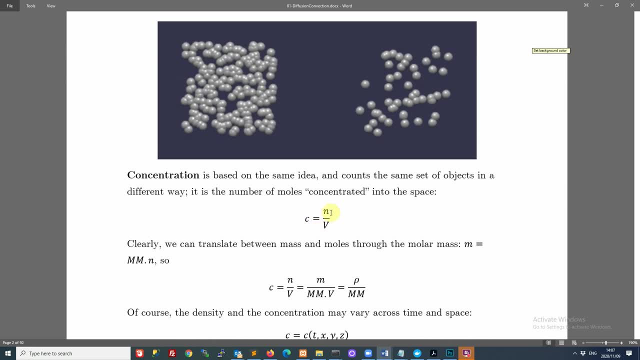 So that's the density of a fluid. And then we can also define the concentration as the number of moles divided by the volume. So in some volume there's some number of moles in that volume. So that number of moles divided by that volume. 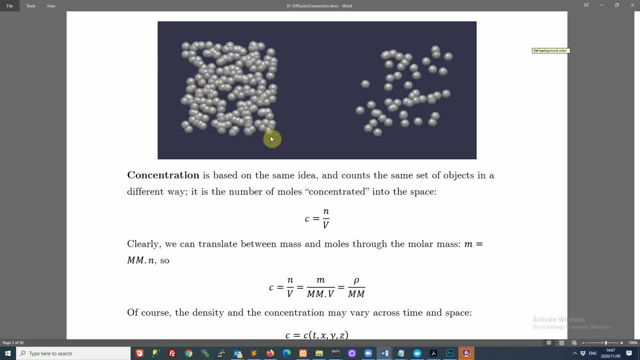 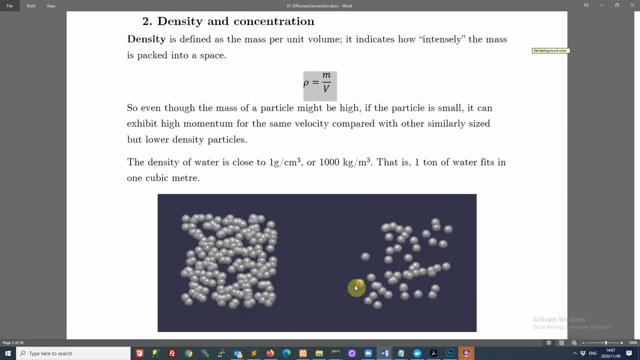 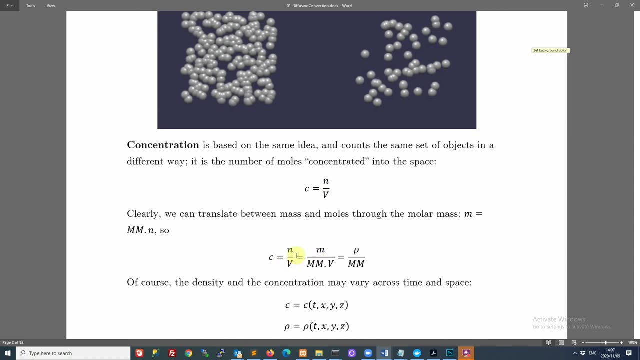 that's an indication of how tightly packed the molecules are in that space. We can translate between concentration and density because, as we said, density was mass of a volume, So concentration is only moles of a volume. So clearly, if you take moles, 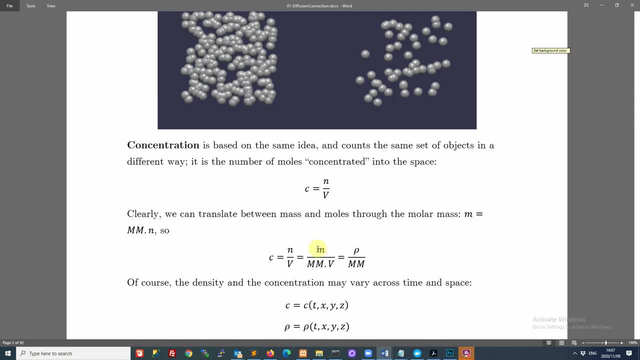 you can rewrite the number of moles in terms of the mass. So if you take the mass and divide by the molar mass, then that will give you the number of moles n. So we can easily translate between the concentration and the density. 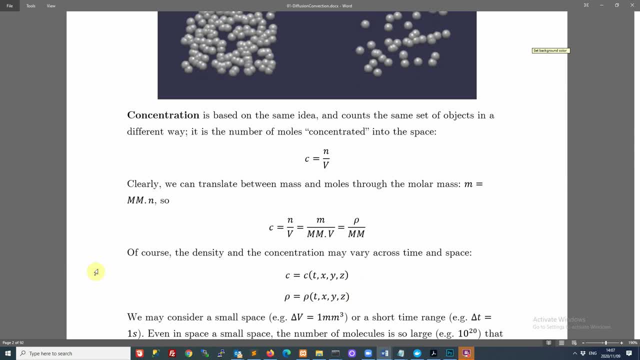 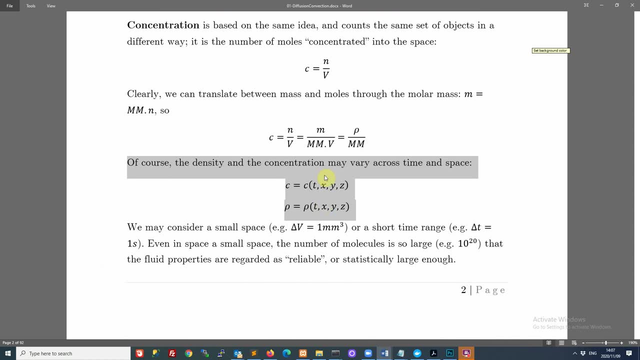 through the molar mass. Now, coming back to what we said about concentration and density varying across time and space, the way we determine this variation is on the understanding that we are free to take a small volume at any point. So let's imagine we take a sampling volume of one cubic millimeter. 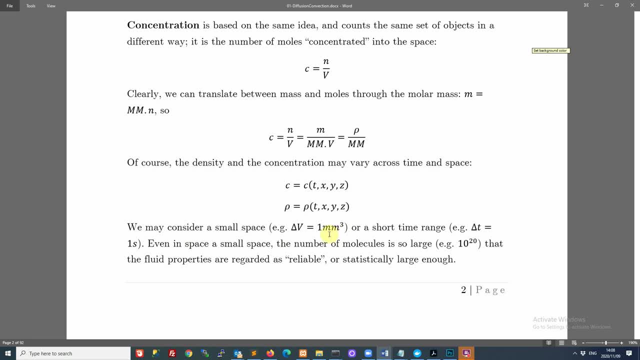 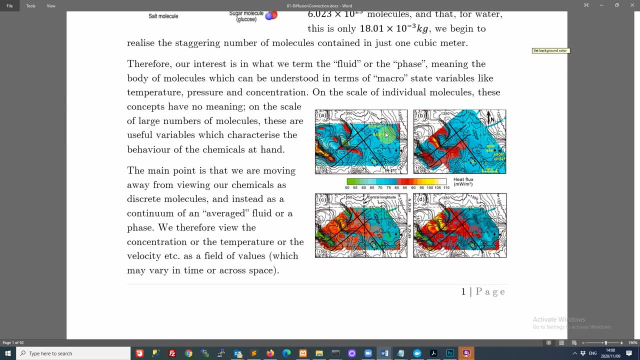 Think about one millimeter and think about, imagine a cube where each side is one millimeter long. Then for example, going back to this weather pattern type example, if we pick some random location, so if we pick, for example, a very specific latitude and longitude, 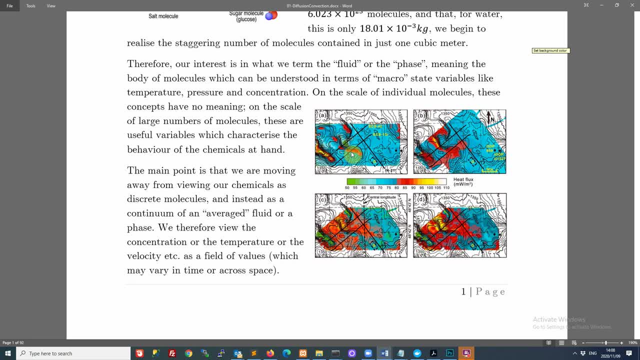 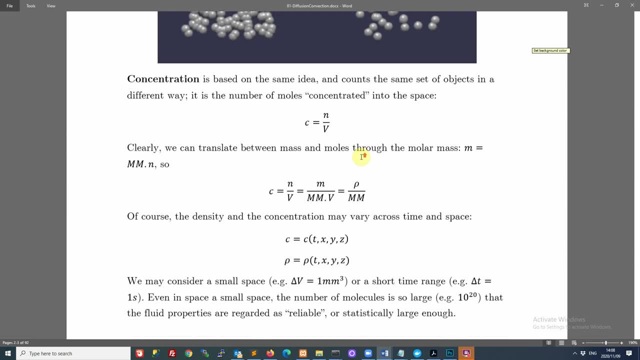 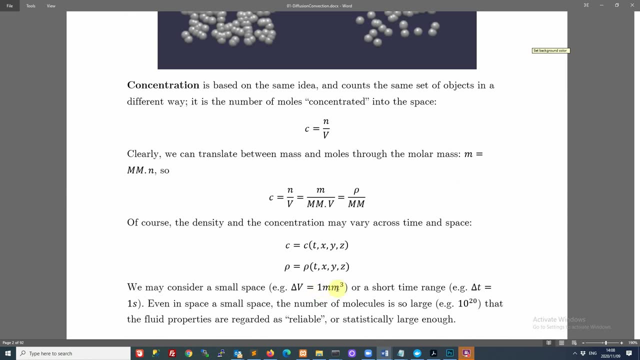 then we can easily imagine taking a sample of just one cubic millimeter in that location. And then we know that even in one cubic millimeter there's still an incredible number of molecules there. It might be on the order of 10 to the power 20 molecules. 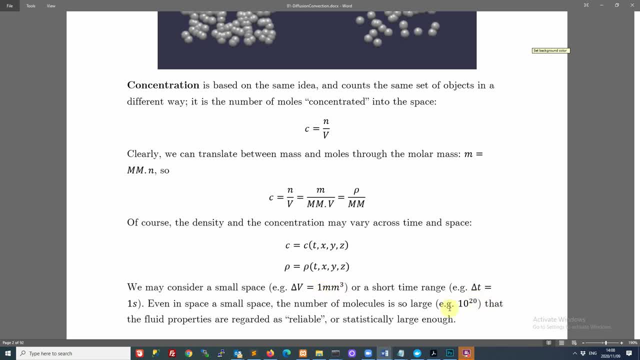 within that one cubic millimeter. And so because there are so many molecules in such a small space, well, in the space of interest, because we have so many molecules, we can say that our estimate of the concentration or the density is going to be quite reliable. 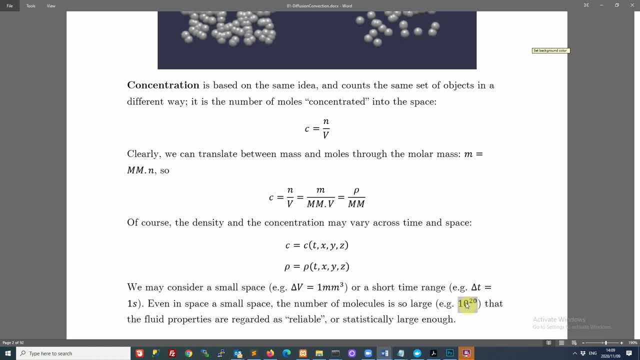 In other words, we have enough molecules in the space, that we have a statistically large enough number of molecules that the way those molecules behave is going to be a good indication of the average property of that fluid. And you see, it's not the case. 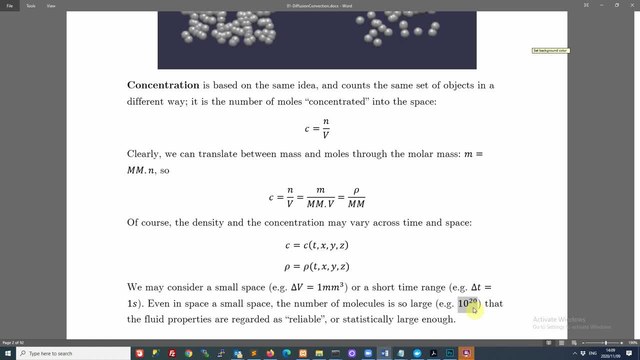 if you had, let's say, two or three molecules. So those two or three molecules, perhaps they are undergoing some kind of chemical change, or if they are not quite the, if they don't have quite the molecular structure that we expect, so there might be some deviation about them. 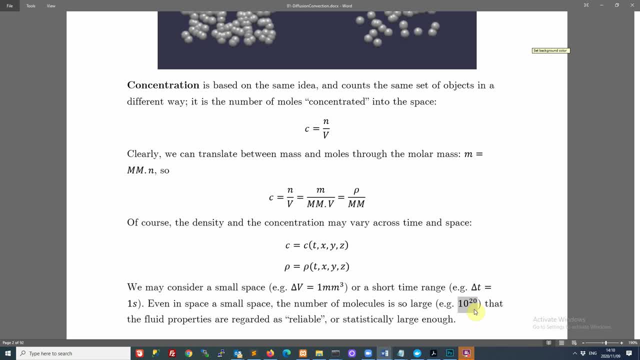 In a very small collection of molecules there might be some deviation that we didn't expect, But if you take such a large number of molecules, such unexpected deviations have a very low probability. In other words, it's a large enough sample even in such a small space. 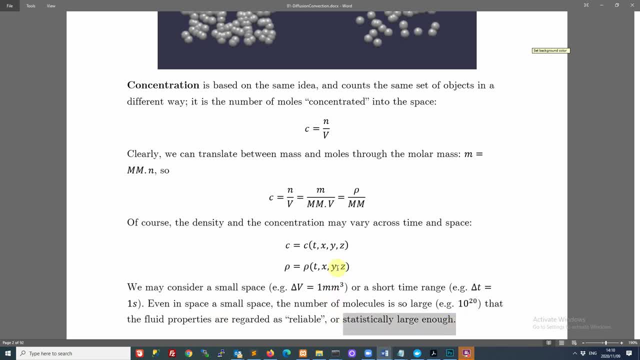 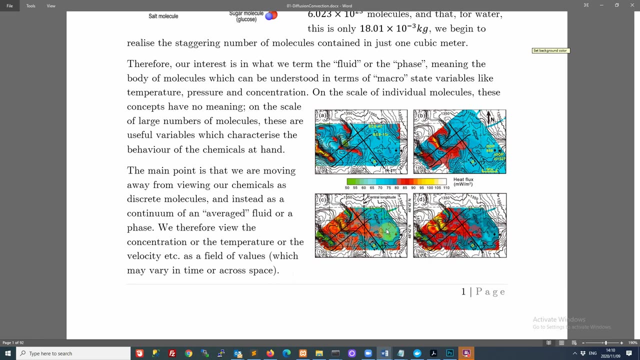 that we can say that if we just find the property in that small space, then that's a good indication of the values of the state in that space. So the whole point of that is to explain how we can get point estimates. So when we talk about the temperature, 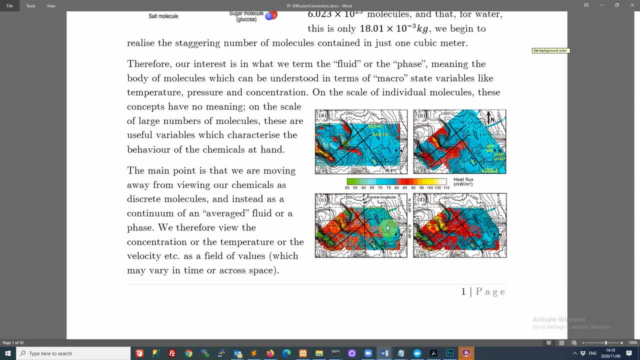 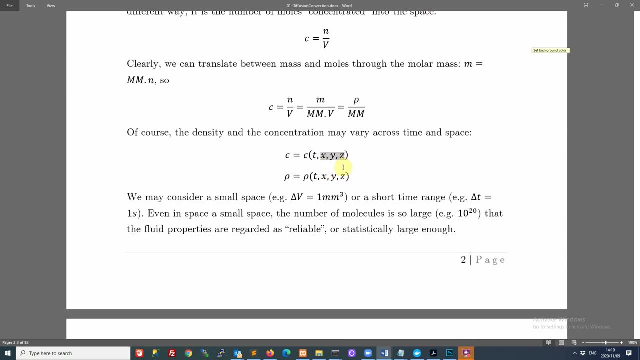 at a specific point, then the understanding is we are taking a small sample at that point. But even small means a very large number of molecules, And so we can easily define the concentration and density at a specific location in our fluid.